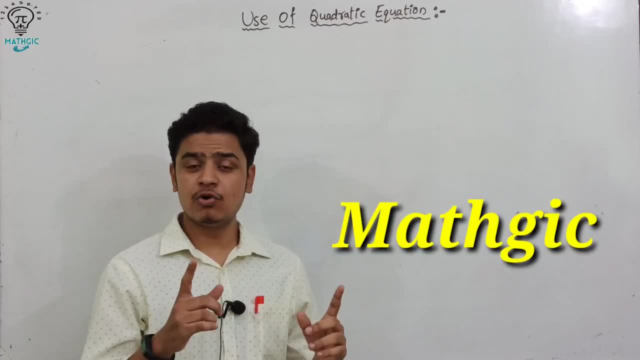 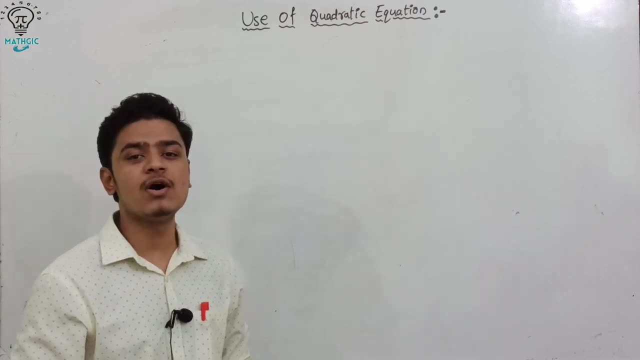 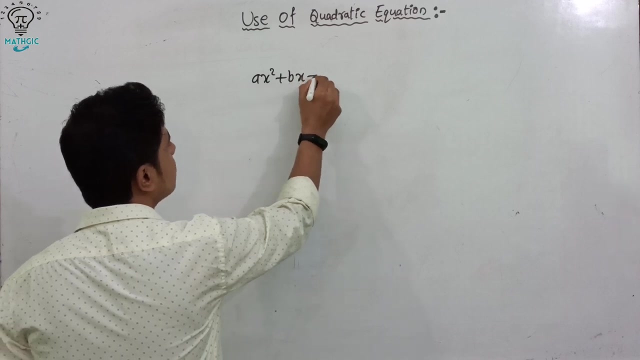 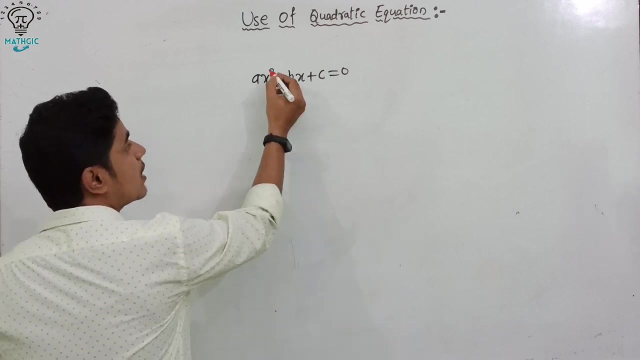 Hello guys, welcome to magic. This video is to understand use of quadratic equation in our day to day life. Before going to that, you should know what is meaning of a quadratic equation. So an equation is of the form: ax square plus bx plus c is equal to zero, is called a quadratic equation. So what make it is quadratic. The power of x is 2. This make a quadratic. So for that, the a 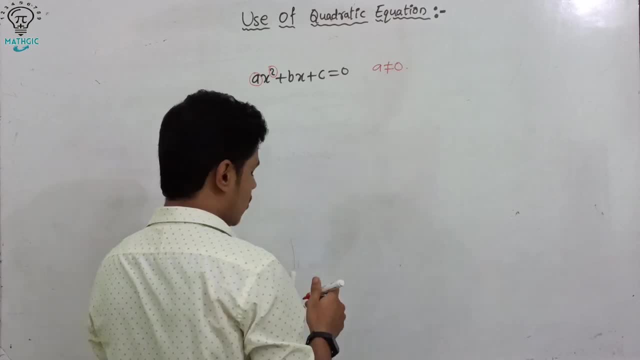 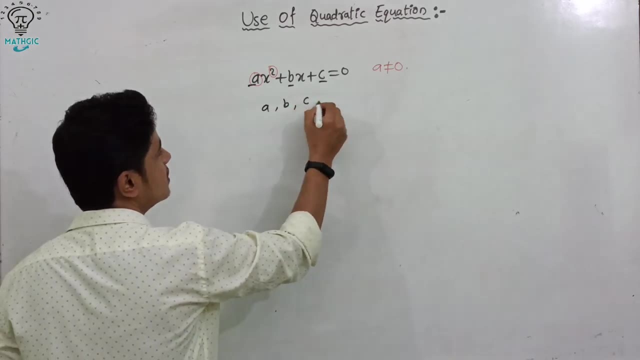 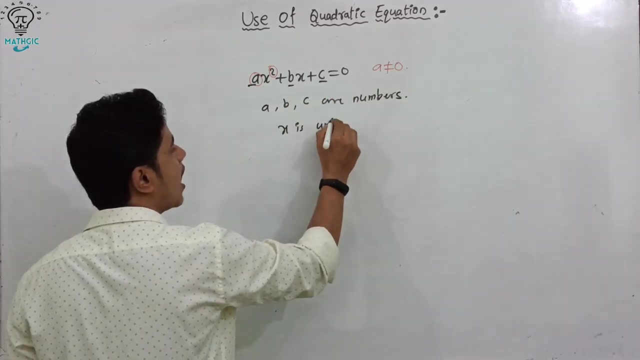 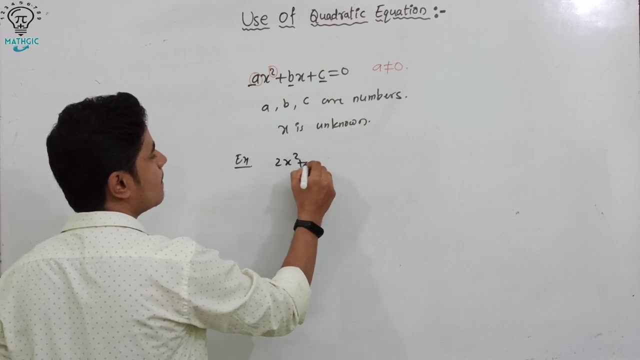 must not be 0. So a should not be equal to zero. What is a and b? So a, b and c are some numbers. a, b, c are numbers, Numbers and x is variable. X is unknown. An example of quadratic equation: an example of quadratic equation: 2xy square plus 5x plus 10 is equal to zero. So these are the example of quadratic. 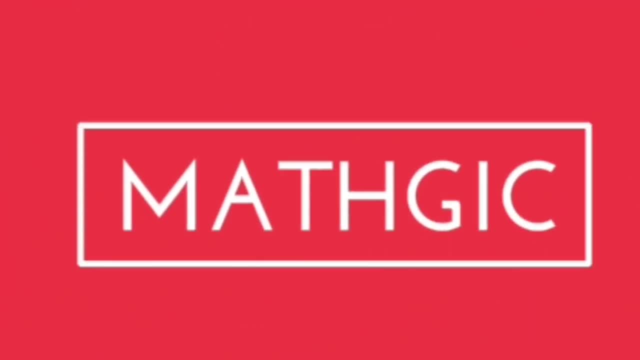 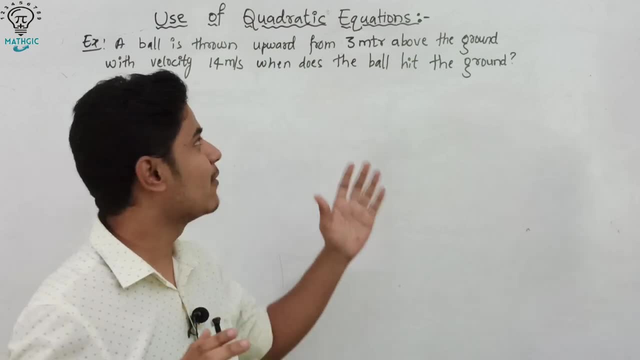 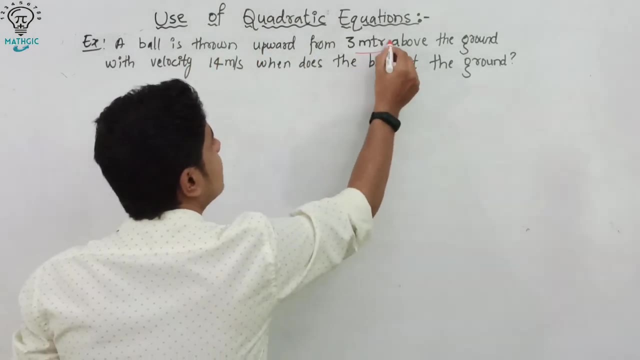 equation. So these are the example of quadratic equation. So these are the example of quadratic equation. So let's get started. Let's have an example of quadratic equation in our day to day life. A ball is thrown upward from a three meter above the ground with a velocity of 14 meter per. 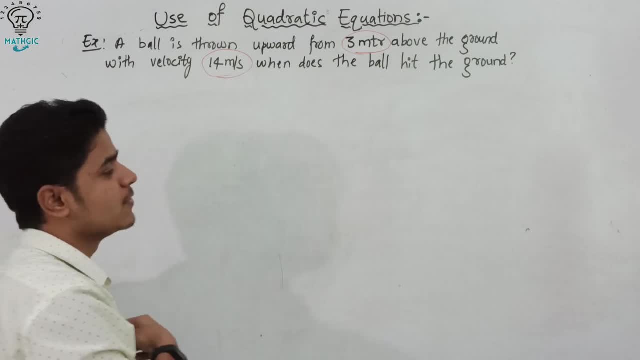 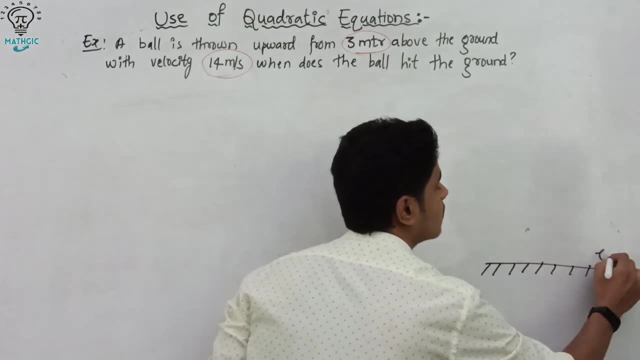 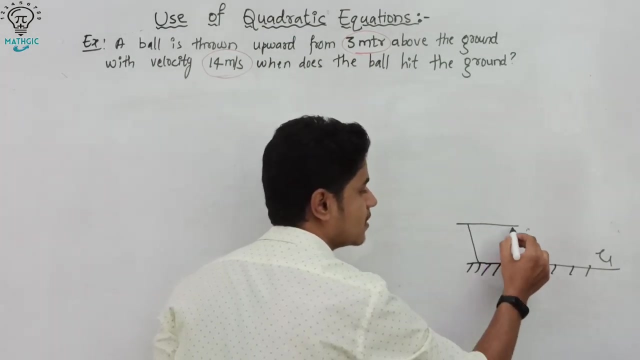 second, We have to find when does the ball reach the ground? So let's draw the diagram for understanding. So this is our ground and the ball is thrown three meter from the ground. So let's have a draw table. That height of the table will be three meter, The ball thrown from a three meter. 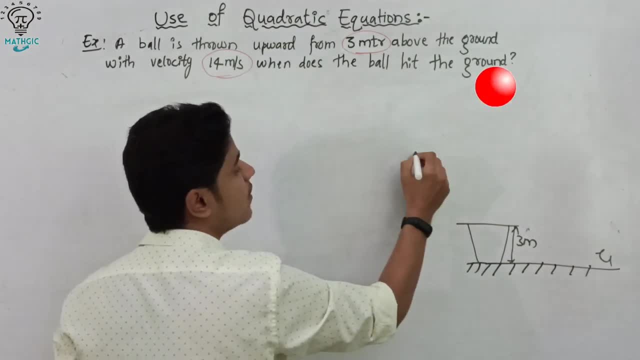 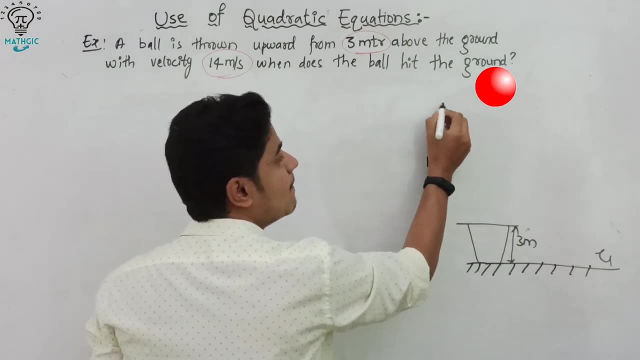 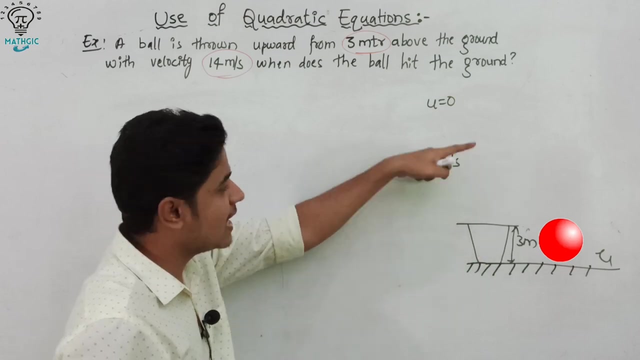 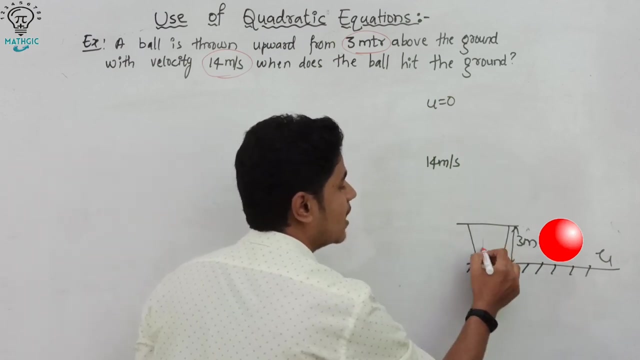 above the ground. So, with a velocity of 14 meter per second and due to the gravity, ball stop at some point, Let's call as initial velocity become a zero. After that the ball getting decreased and reach the ground. We have to find that time, So let this distance called as a d1 distance from ground and 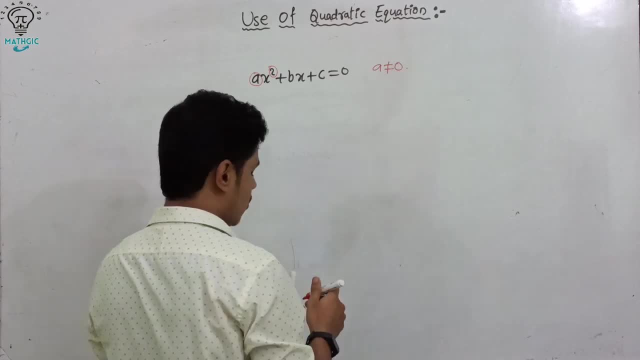 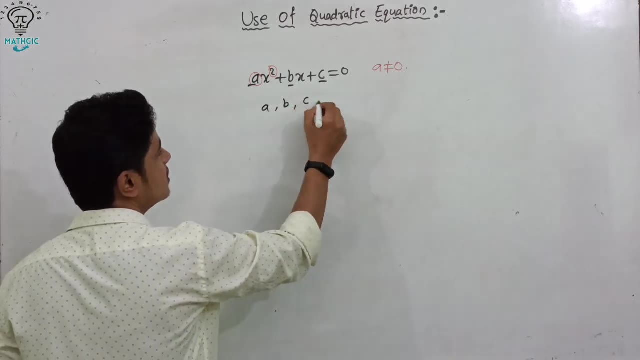 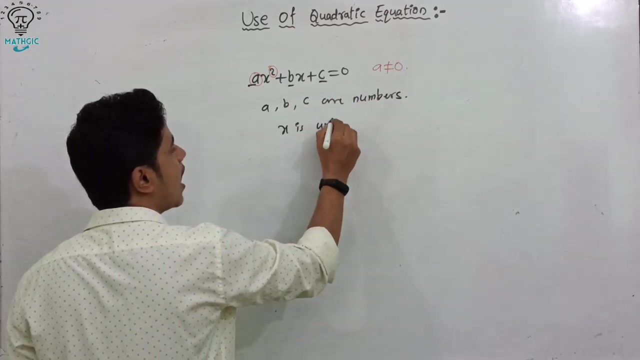 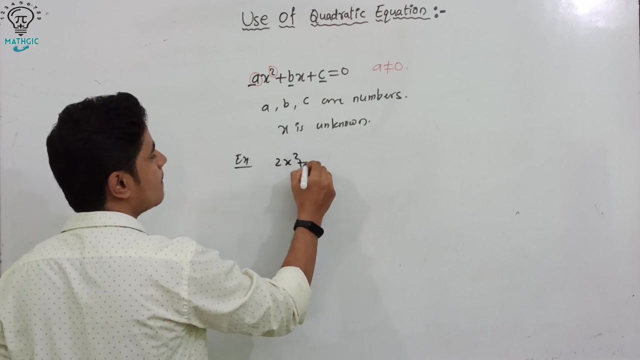 must not be zero, So a should not be equal to zero. What is a and b? So a, b and c are some numbers. a, b, c are numbers, Numbers and x is variable. x is unknown. An example of quadratic equation: an example of quadratic equation: 2x square plus 5x plus 10 is equal to zero. So these are the example of. 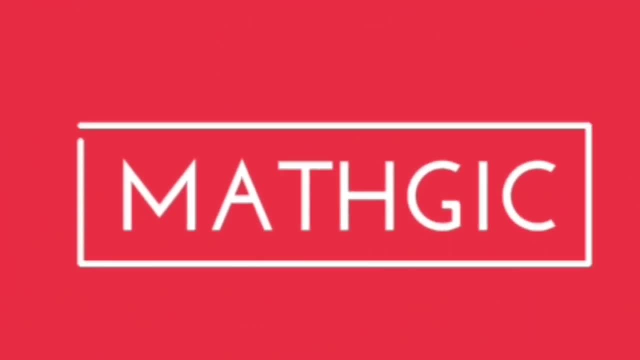 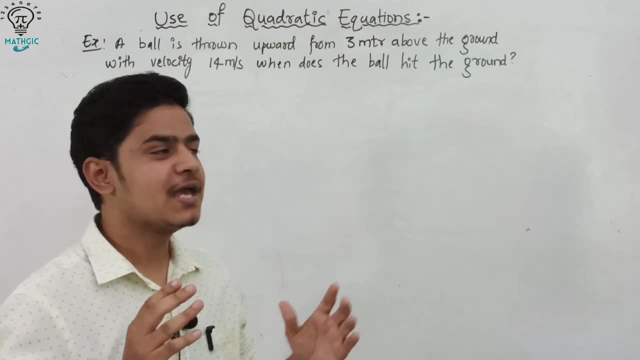 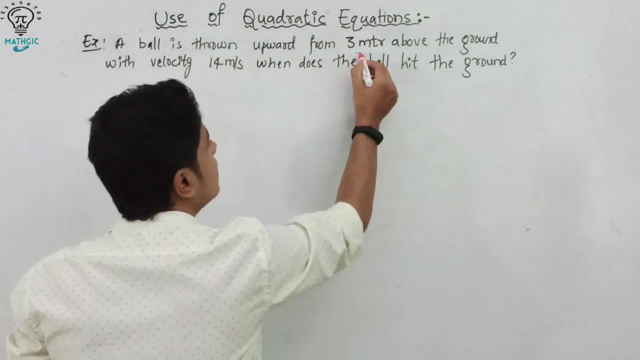 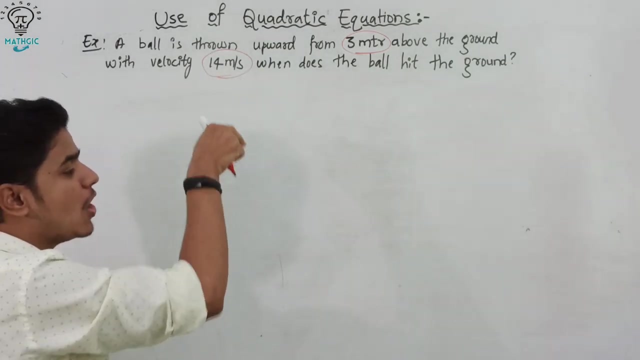 quadratic equation- equation. So let's get started. Let's have an example of quadratic equation in our day to day life. A ball is thrown upward from a three meter above the ground with a velocity of 14 meter per second. We have to find: when does the ball reach the ground? So let's draw the diagram for. 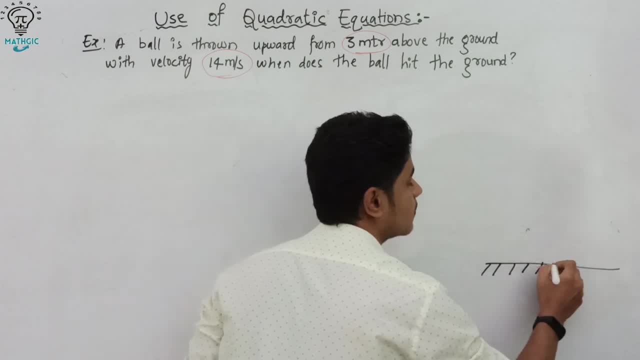 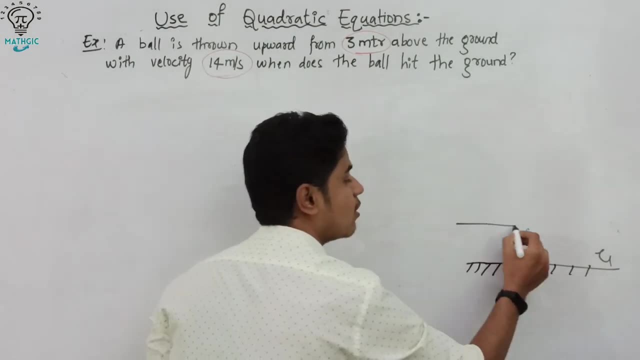 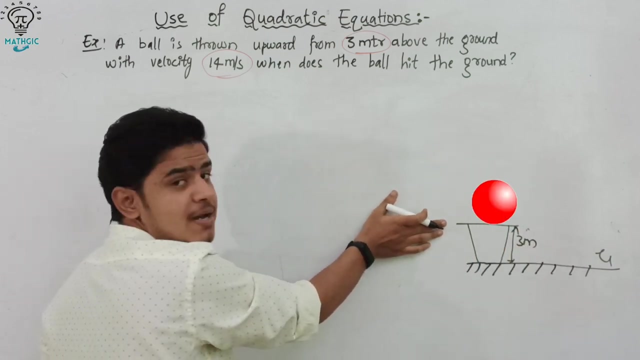 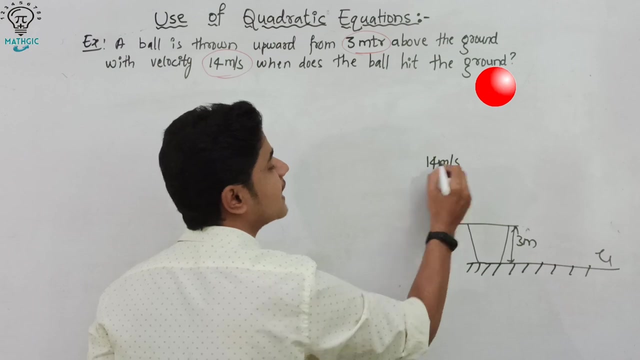 understanding. So this is our ground and the ball is thrown three meter from the ground. So let's have a draw table. That height of the table will be three meter, The ball thrown from a three meter above the ground, So with a velocity of 14 meter per second and, due to the gravity ball, stop at. 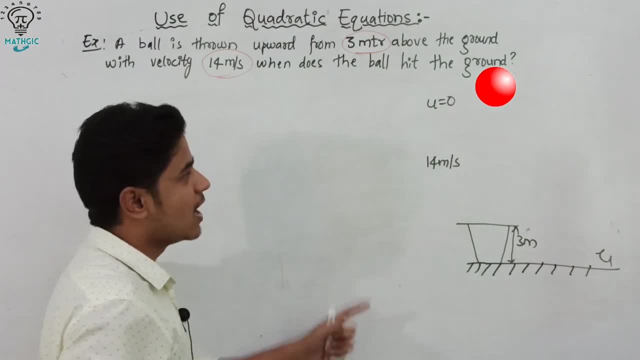 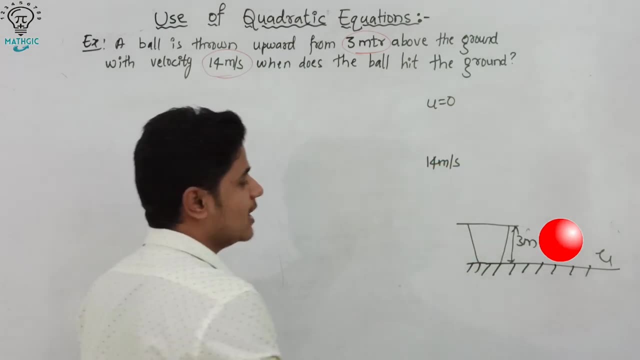 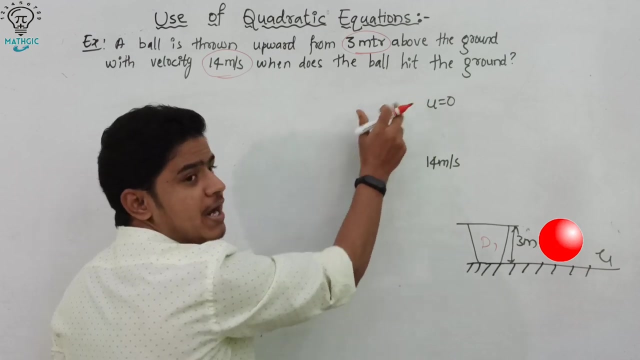 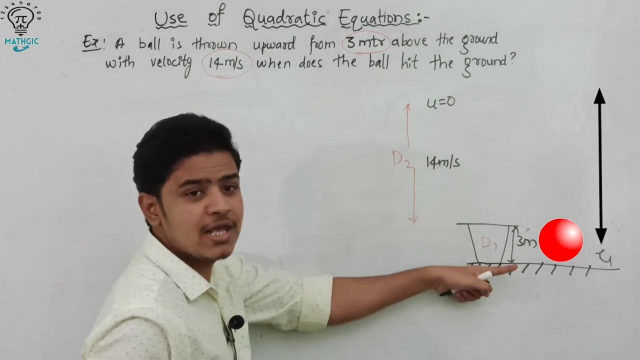 some point- Let's call as initial velocity- become a zero. After that the ball getting decreased and reach the ground. We have to find that time. So let this distance called as a d1 distance from ground and table d1 and from this table point where ball stop d2, where ball stop d2, and from top to the bottom. 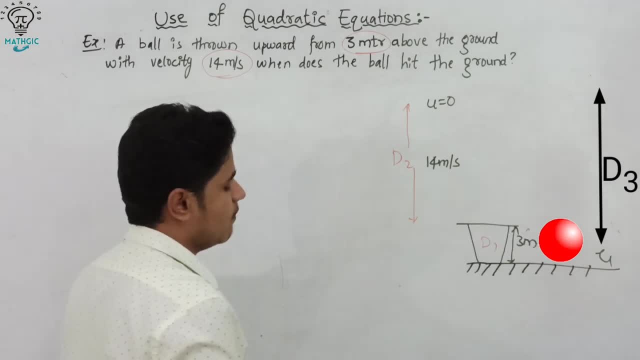 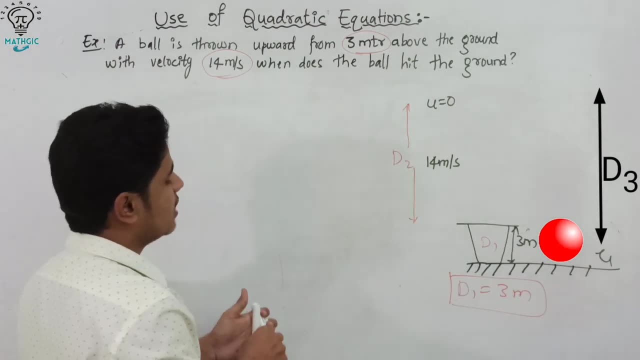 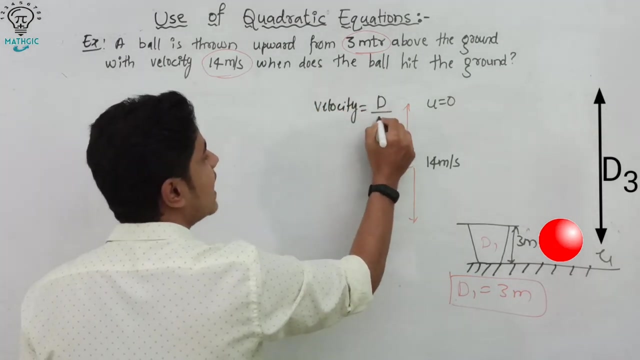 where ball hit the ground, that is d3.. So first of all we have to find: d1 is equal to three meter and D two. So the velocity is equal to. velocity is equal to displacement by time. T velocity is 14 meter. Fourteen is equal. 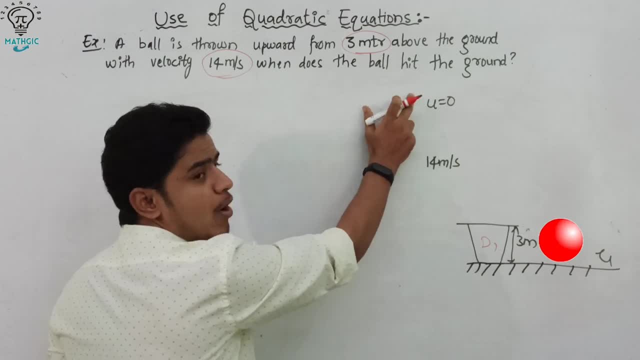 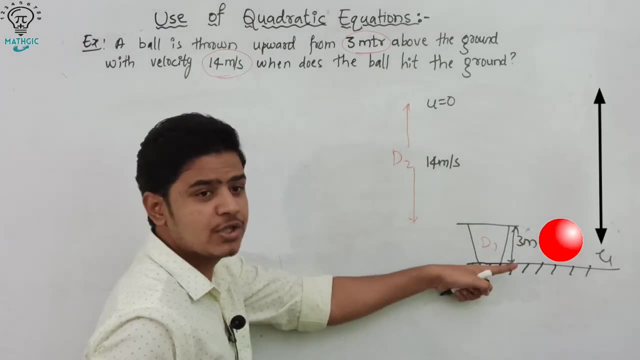 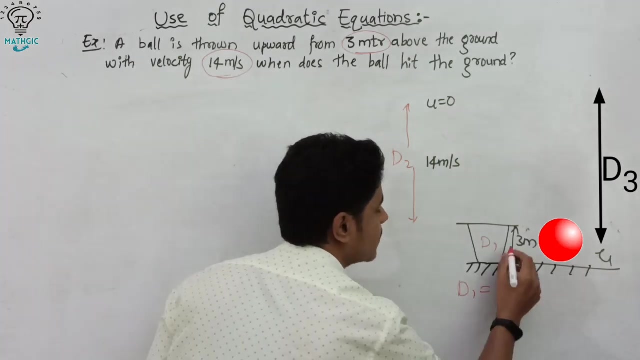 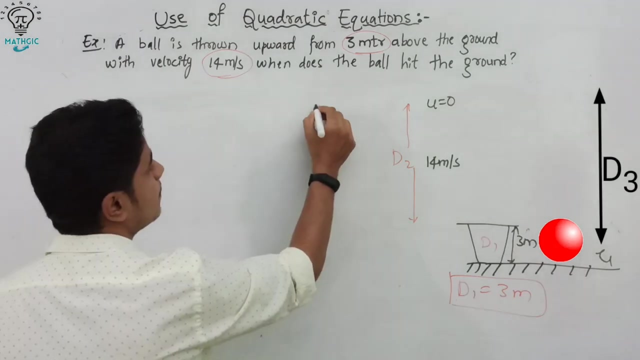 table d1 and from this table point where ball stop d2, where ball stop d2, and from top to the bottom where ball hit the ground, that is d3. So first of all we have to find d1 is equal to three meter and have to find d2.. So the velocity: velocity is equal to, velocity is equal to. 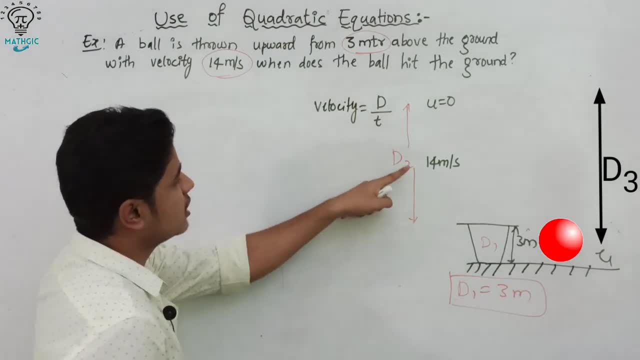 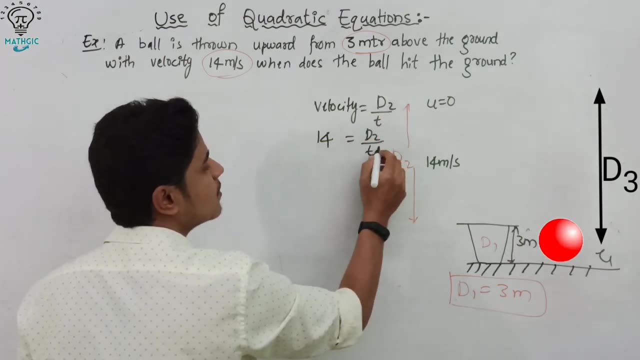 displacement by time. t velocity is 14 meters. 14 is equal to the distance, it d2.. And d 2 divided by time. So we have to find d2, multiply time t, both side t tr. cancel It willpolitik 14 t. 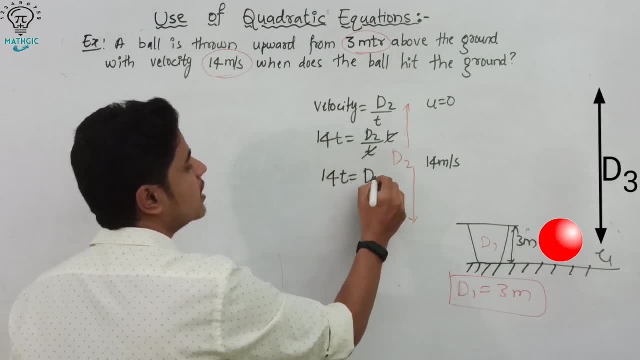 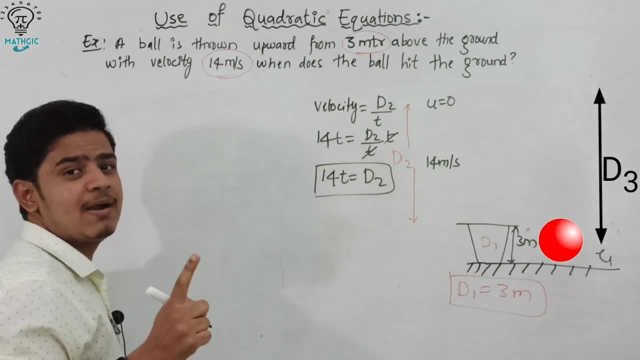 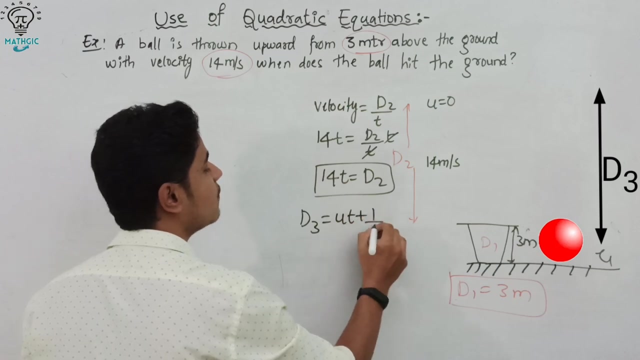 14 t. t is equal to distance d2.. So d2 will be 14t and to find d3.. So there is a relation between initial velocity and acceleration, that is distance. d3 is equal to u into t plus half of a into t. 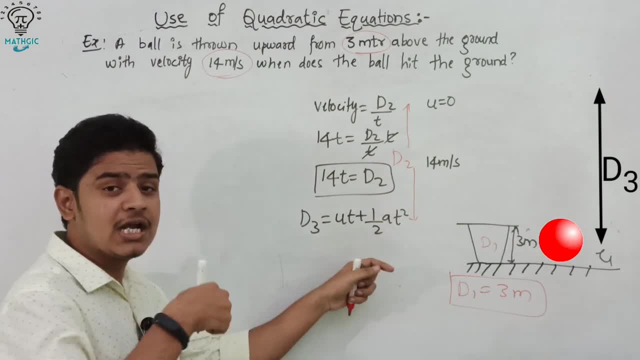 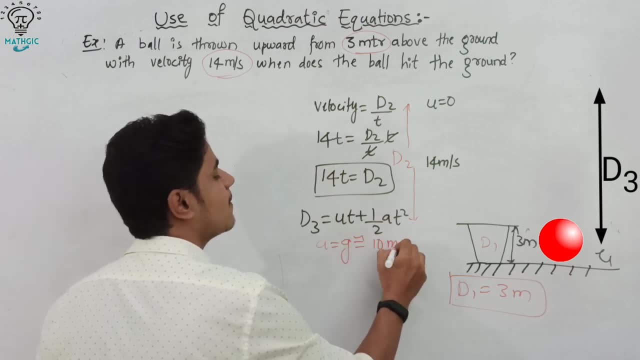 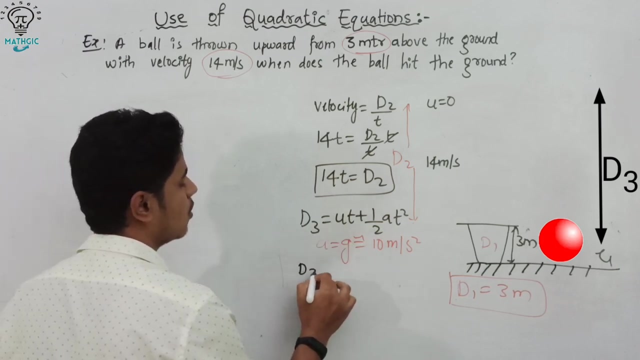 square. Here u is initial velocity and a is acceleration due to the gravity error. So now the constant value of a, that is, acceleration due to the gravity, is 10 meter per second square, Or sometime taken as 9.8 meter per second square. Let's substitute here, So d3 is equal to u is 0. 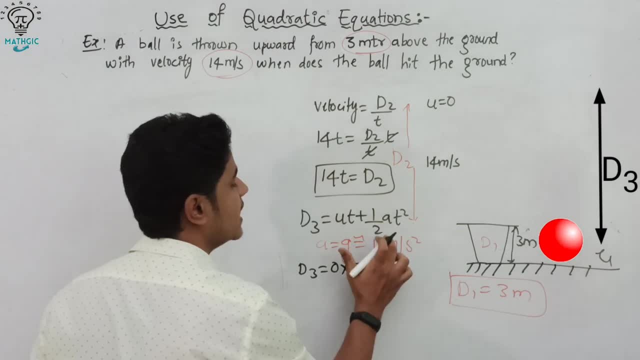 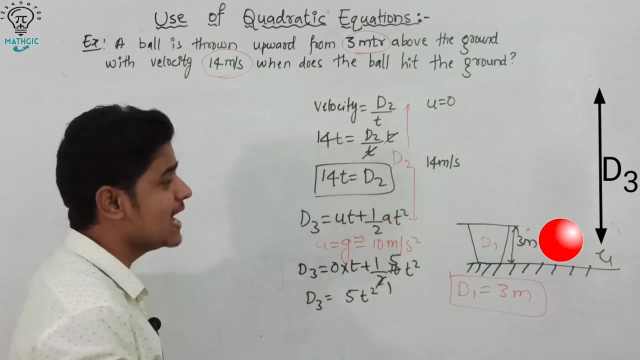 into t plus 1 by 2 a is 10 t square, 2 1 z to 5 z 10.. So 5 t square, 5 t square. this is your d3.. But the direction when ball come, returning to the ground that is a opposite to the starting. So 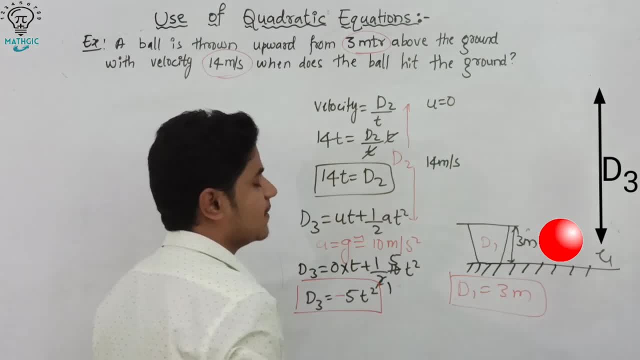 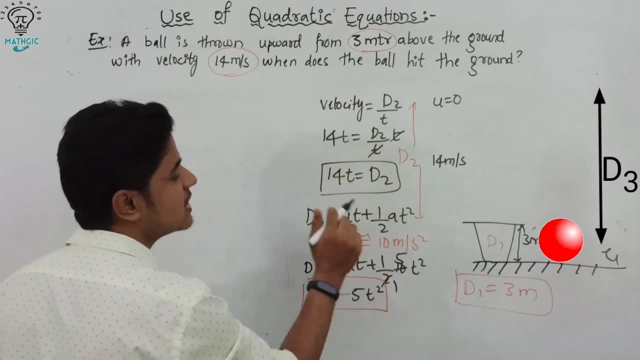 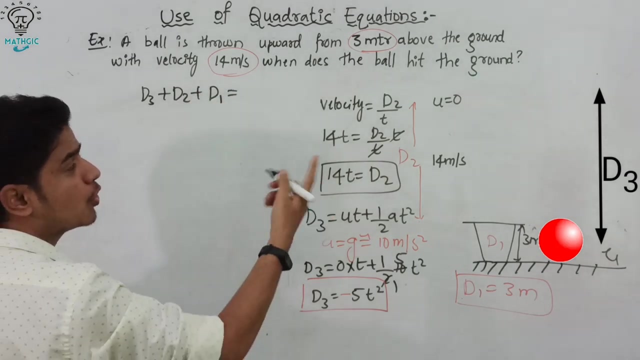 this should be minus. So this is Cover d3.. So the total distance covered by ball in all is d3 plus d2 plus d1. So that is d3 plus d2 plus d1 is equal to total distance covered by ball is considered d. So now d3 is minus 5t. 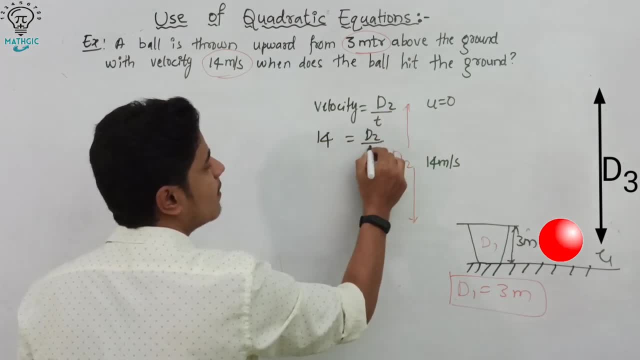 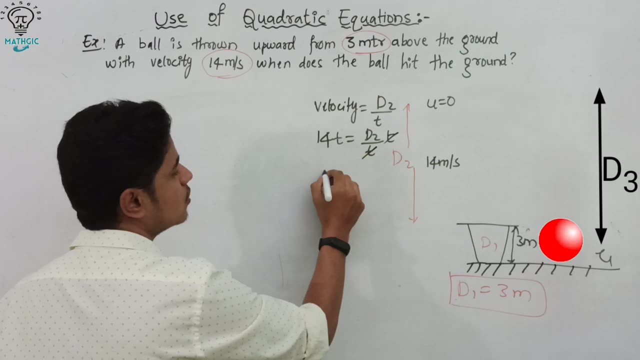 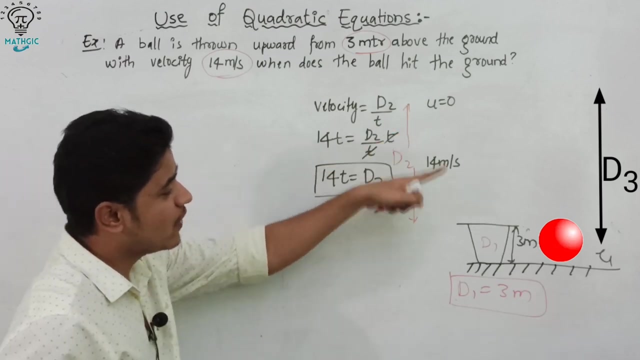 to the distance is D two And D two divided by time. to find d2, multiplied by time, both side, T, T, t, cancel, and after 14, 14t is equal to distance d2. So d2 will be 14t And to find d3, so there is a relation. 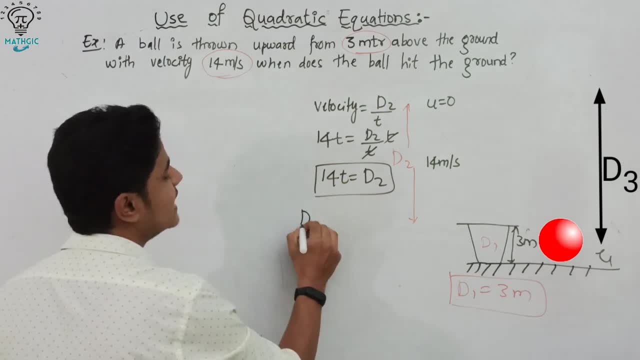 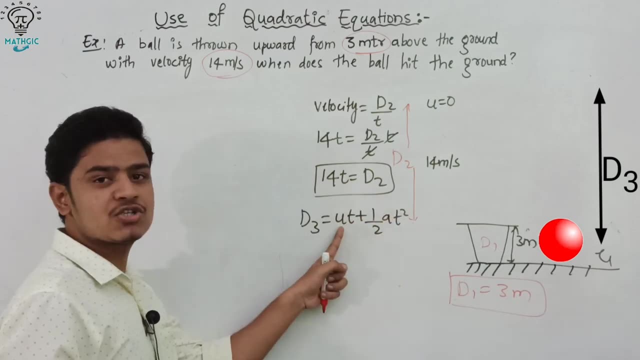 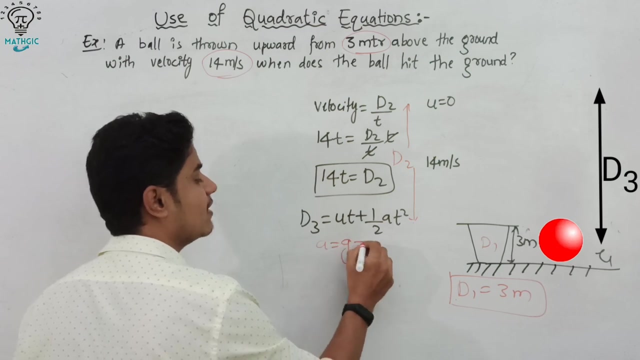 between initial velocity and acceleration, That is distance. d3 is equal to u into t plus half of a into t square. Here u is initial velocity and a is acceleration due to the gravity. here So now the constant value of a, that is acceleration due to the gravity. 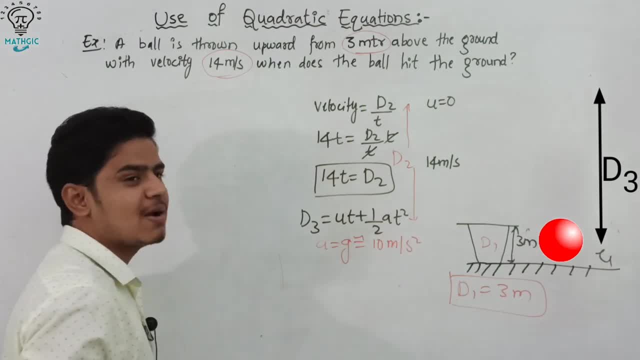 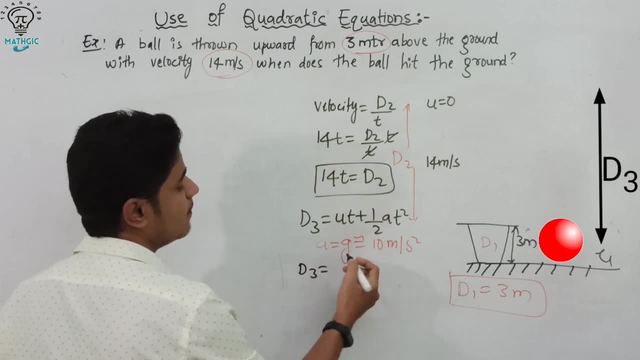 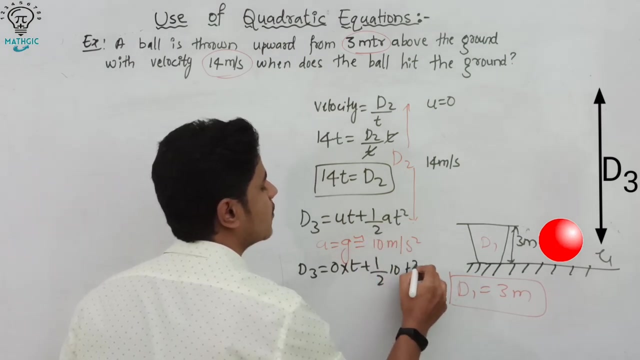 is 10 meter per second square or sometime taken as 9.8 meter per second square. Let's substitute here. So d3 is equal to: u is 0 into t plus 1 by 2, a is 10, t square 2: 1. 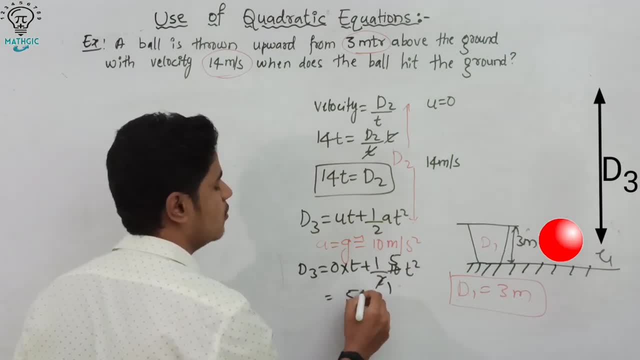 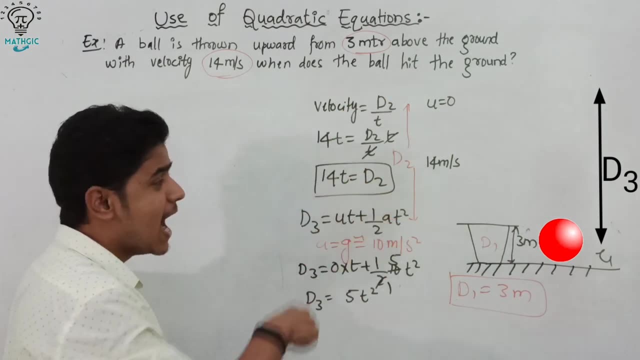 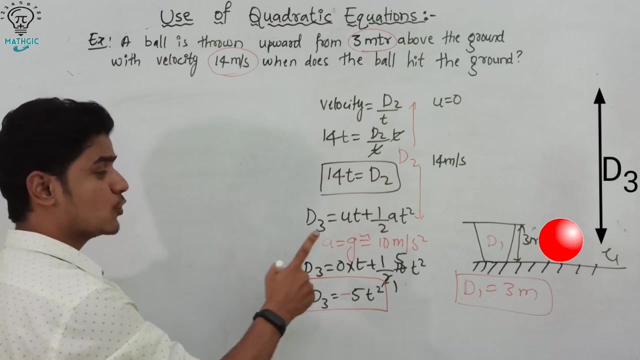 z to 5 is 10.. So 5t square, 5t square, this is your d3.. But the direction when ball come, returning to the ground that is a half Opposite to the starting, So that is should be minus. So this is our d3.. So the total 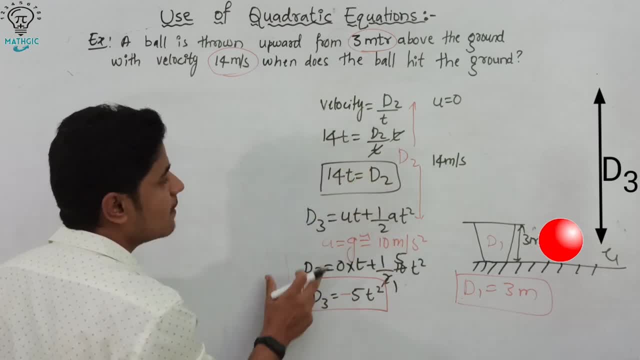 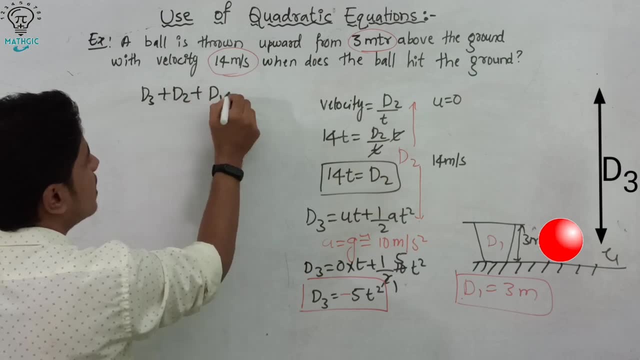 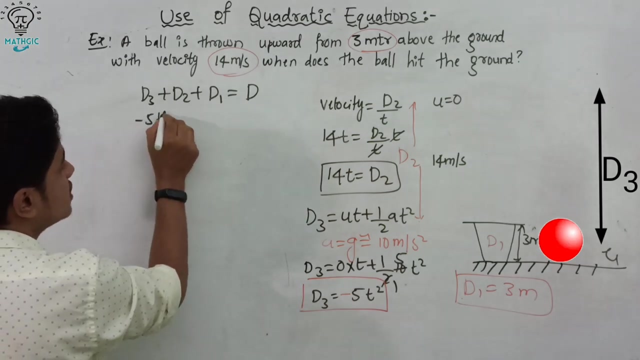 distance covered by ball in all is d3 plus d2 plus d1.. That is d3 plus d2 plus d1 is equal to total distance covered by ball. is considered d? So now d3 is minus 5t, minus 5t. square plus d2 is 14t plus d1.. 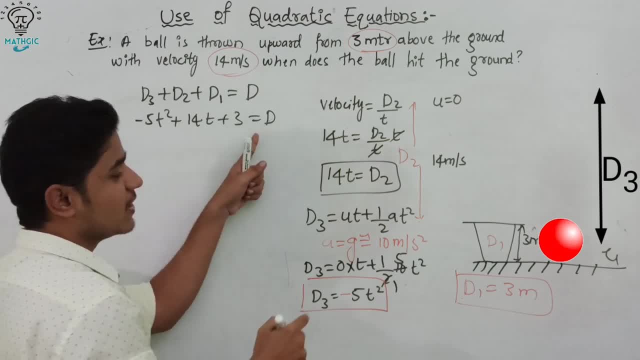 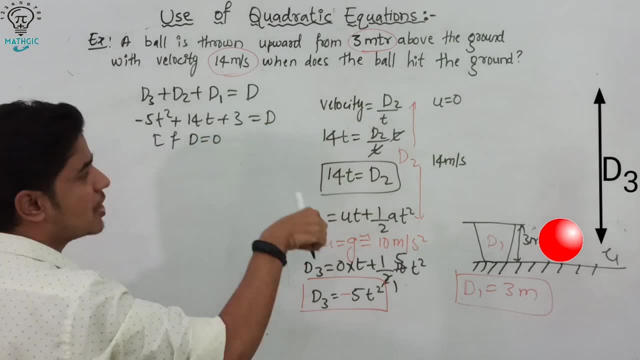 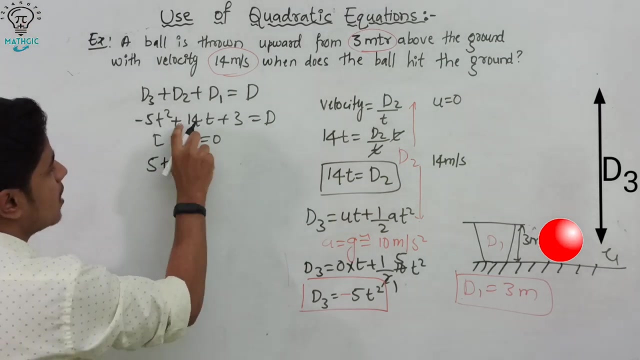 d1 is 3 is equal to d. If the distance is become 0, then the ball reach the ground. If d equal to 0, ball return the ground. Now substitute: So take minus 5, common here. So minus common. So minus minus plus 5t square, minus plus minus 14t minus 3 is equal to 0. 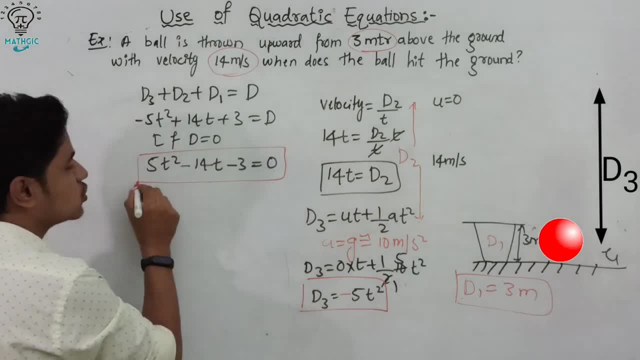 So this is the form of a quadratic equation: We have to solve for t to get a square. So this is the form of a quadratic equation: We have to solve for t to get a square. So this is the form of our solution. where t is time. Let's see how to solve This method. 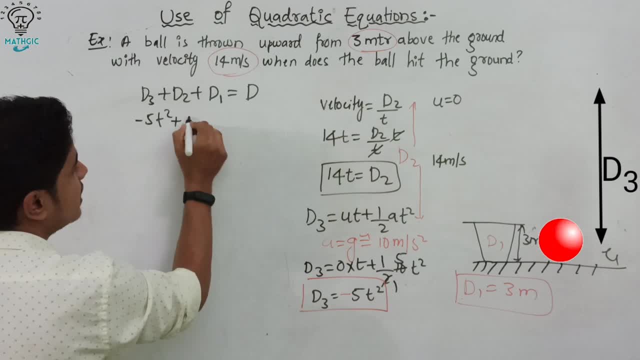 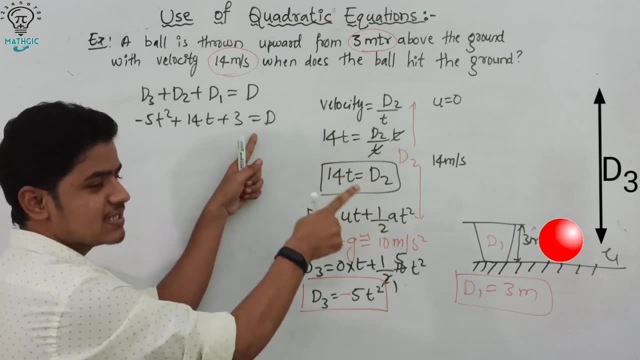 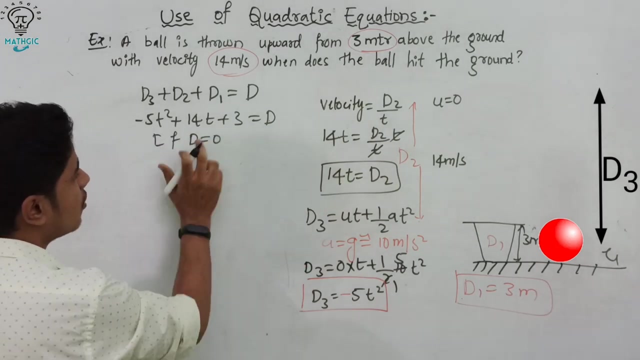 minus 5t square plus d2 is 14t, plus d1 is 3 is equal to d. If the distance is become 0, then the ball reach the ground. If d equal to 0, ball return the ground. Now substitute: So: take minus 5 common here, So minus common. So minus minus plus 5t square. 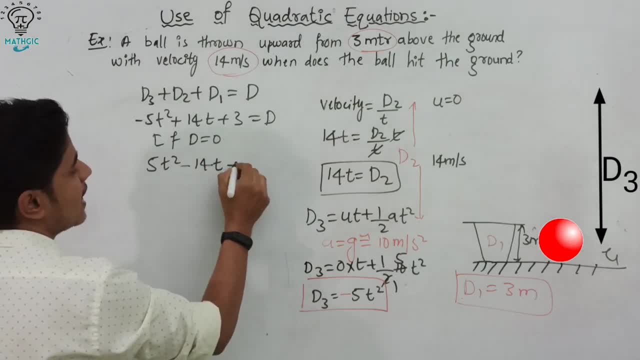 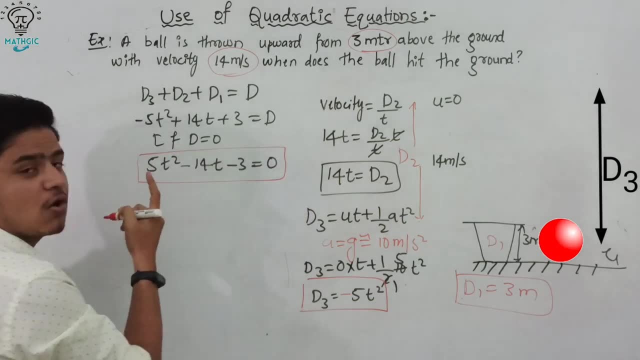 minus plus minus 14t minus 3 is equal to 0. So this is the form of a quadratic equation. We have to solve for t to get a solution where t is a time. So let's see how to solve This. 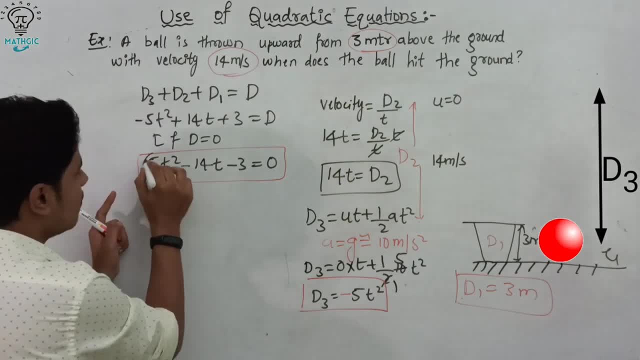 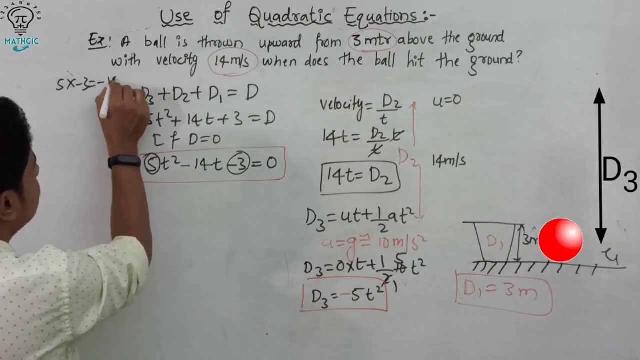 method is called as a factorization method. So now multiply 5 and minus 3.. So 5 into minus 3 is equal to minus 15.. Now choose the factor of 15.. Choose the factor of 15.. If you multiply, you should. 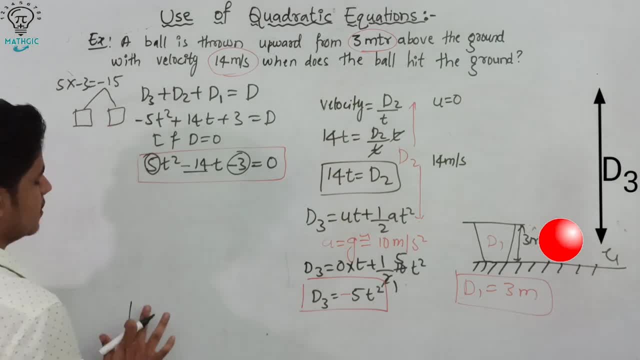 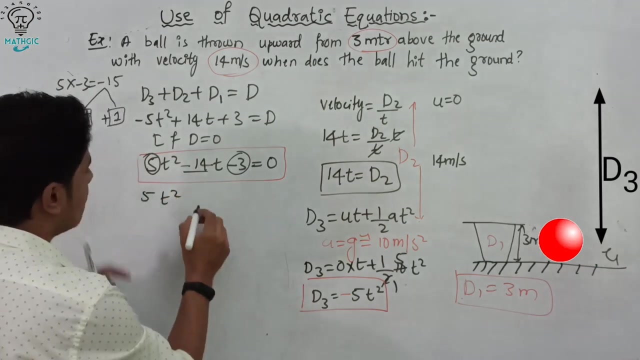 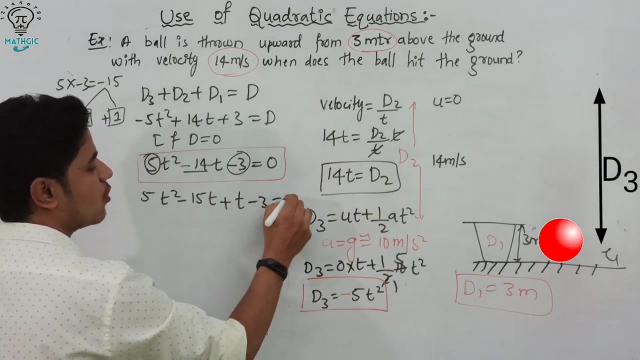 get 15, and if you add or subtract you should get minus 14.. So those are 15, ones are 15.. So minus 15 plus 15.. 1. Now substitute In place of minus 14.. 5t square minus 15t plus 1t minus 3, equal to 0.. Now factorize. 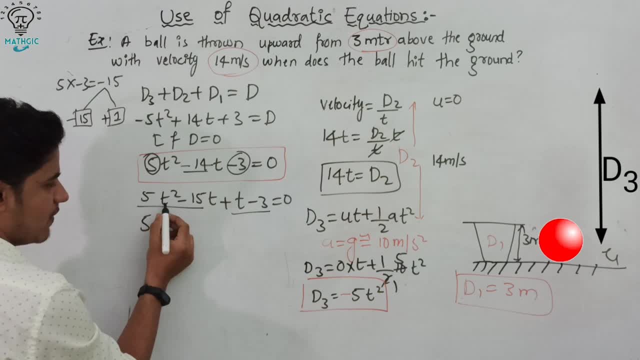 The common factor of 5 and 15 is 5 and common factor of t square and t is t. Divide 5t from 5t square, That is t minus 15t and 5t 3.. Now, plus, There is a common factor of only a, 1.. t minus 3 equal to 0.. So we get only one common factor. 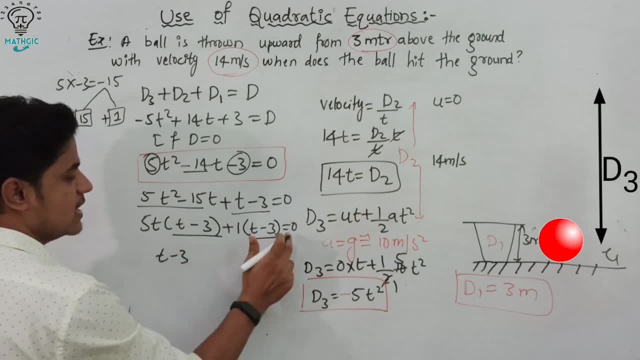 t minus 3.. t minus 3.. So t minus 3 is equal to 0.. Another factor is 5t plus 1.. 5t plus 1 is equal to 0. Here add both side by 3 to get t. So t is equal to 3 in second To time in second. Now here: 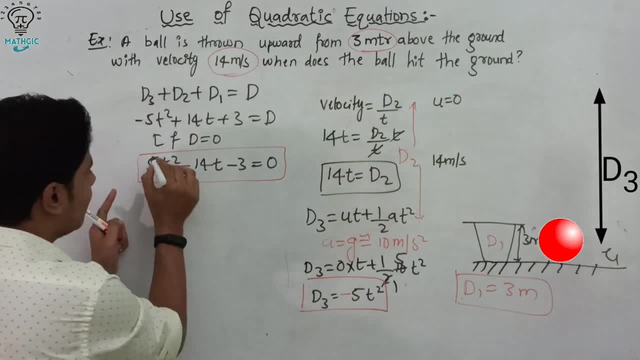 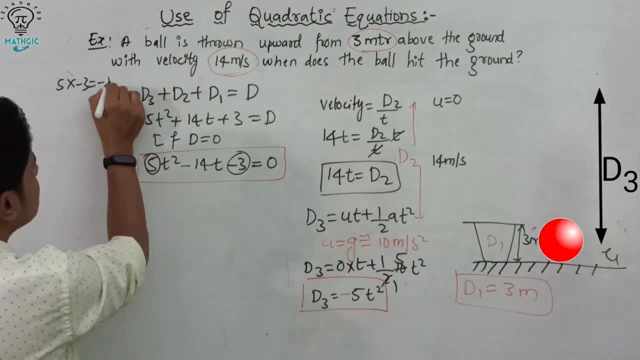 is called as a factorization method. So now multiply 5 and minus 3.. So 5 into minus 3 is equal to minus 15.. Now choose the factor of 15.. Choose the factor of 15.. If you multiply, 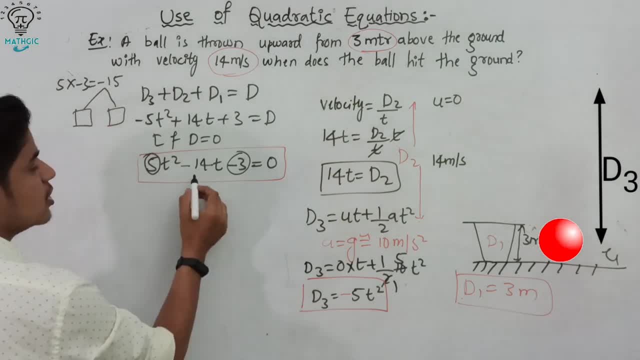 you should get 15.. And if you add or subtract you should get minus 14.. So those are 15, ones are 15.. So minus 15 plus 1.. Now substitute in place of minus 14. 5t square minus 15t plus. 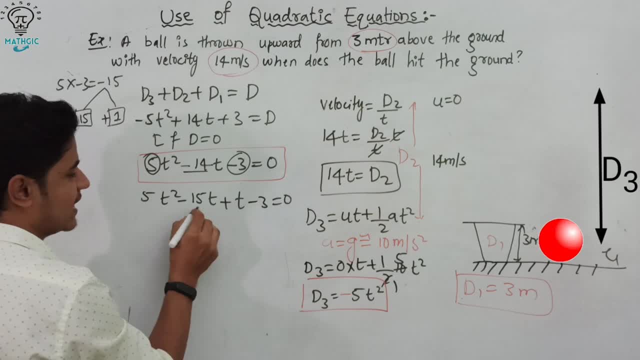 1t minus 3, equal to 0.. Now factorize: The common factor of 5 and 15 is 5 and common factor of t square and t is t. Divide 5t from 5t square, That is t minus 15t and 5t. That. 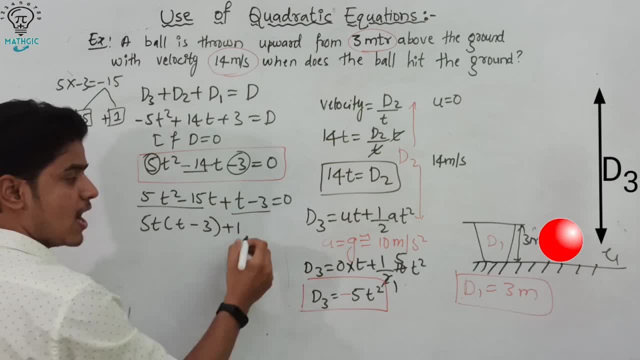 is 3.. Now, plus, There is a common factor only of 1.. t minus 3, equal to 0. So we get only one common factor: t minus 3.. t minus 3. So t minus 3 is equal to 0.. And another factor: 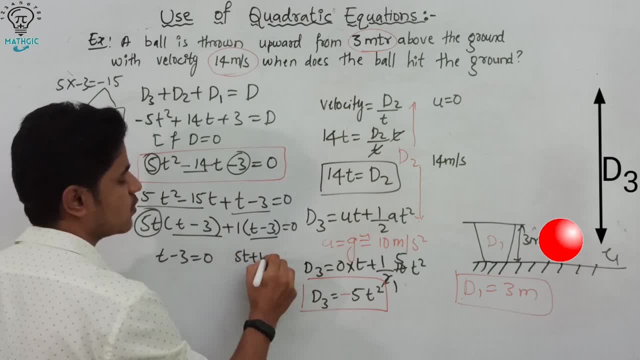 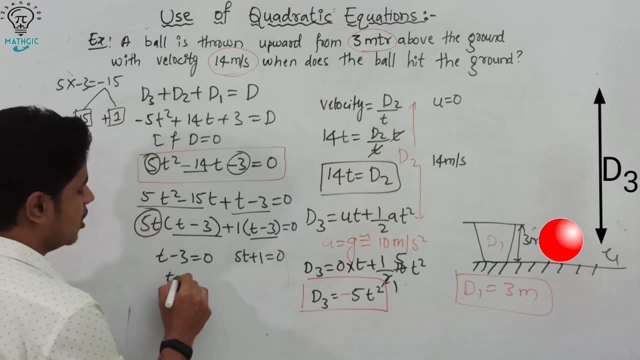 is 5t plus 1.. 5t plus 1 is equal to 0.. Here add both side by 3 to get t, So t is equal to 3. in second Time, in second Now: here subtract minus 1 from both side and divide 5 to get t, So t is equal to minus 1 by 5.. 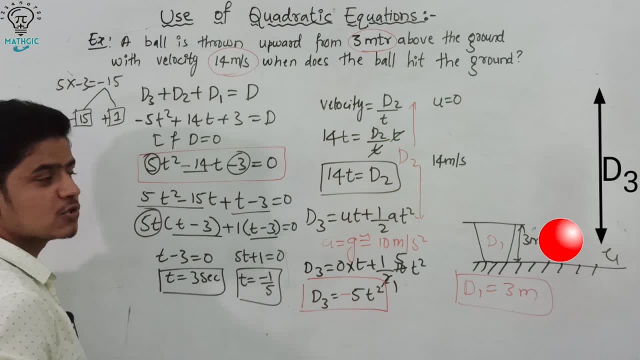 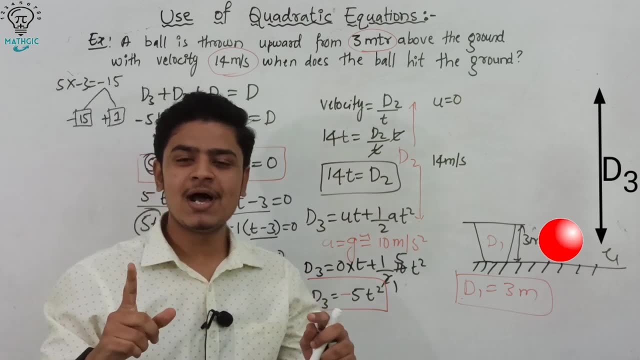 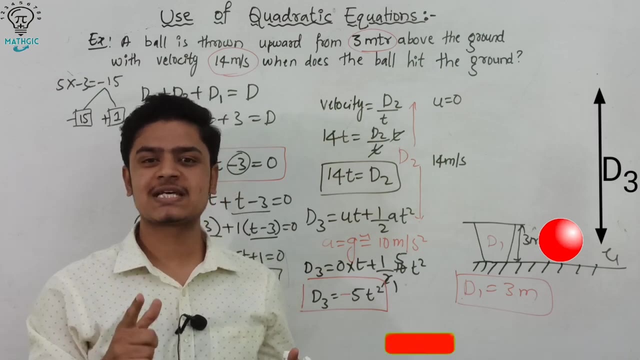 But time should be in positive. So the time when the ball return to the ground is 3 second. So this is the Only one application of a quadratic equation. Hope you understand and like the video. So for more videos, subscribe and press the bell icon so that you can get the notification.